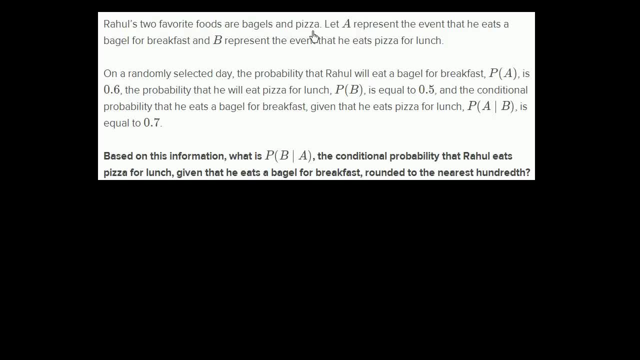 Rahul's two favorite foods are bagels and pizza. Let A represent the event that he eats a bagel for breakfast and let B represent the event that he eats pizza for lunch. Fair enough, On a randomly selected day, the probability that Rahul will eat a bagel for breakfast? 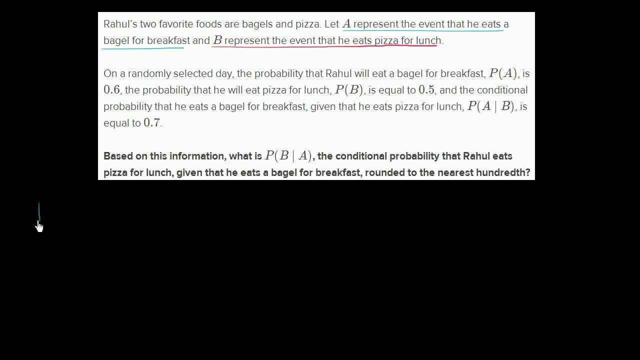 probability of A is 0.6.. Let me write that down. So the probability that he eats a bagel for breakfast is 0.6.. The probability that he will eat a pizza for lunch: probability of event B. so the probability of. 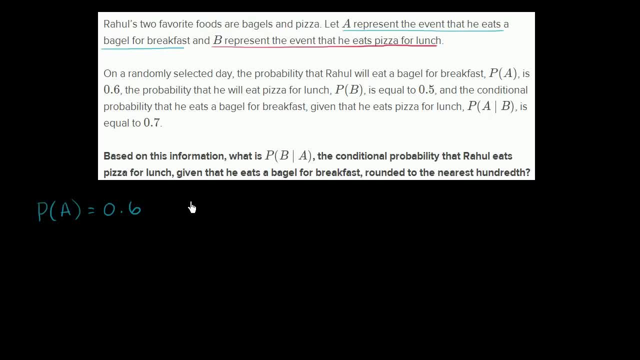 let me do that in that red color. the probability of event B that he eats a pizza for lunch is 0.5.. And the conditional probability that he eats a bagel for breakfast. given that he eats a bagel for breakfast, 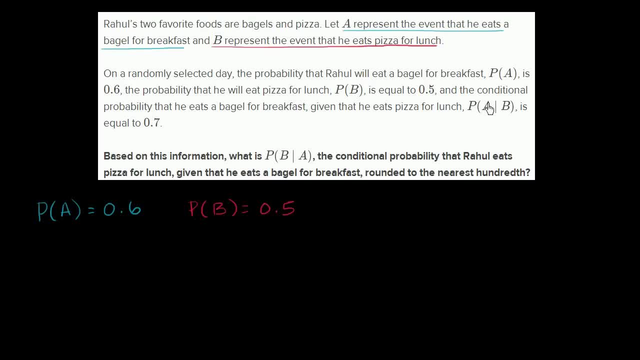 is a pizza for lunch, so probability of event A happening that he eats a bagel for breakfast, given that he's had a pizza for lunch, is equal to 0.7, which is interesting, So let me write this down. 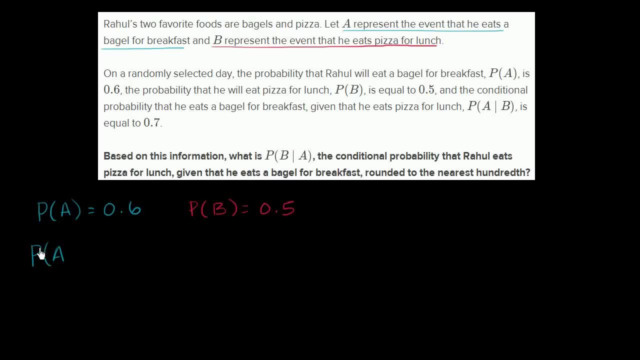 The probability of A, given that B is true, given B is not 0.6, it's equal to 0.7.. And because these two things are not the same, because probability of A by itself is different than the probability of A. 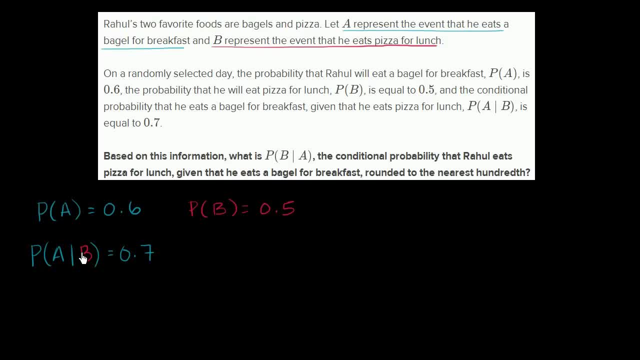 given that B is true. this tells us that these two events are not independent, that we're dealing with dependent probability. This shows us the fact that B being true has changed the probability of A being true. This tells us that A and B are dependent. 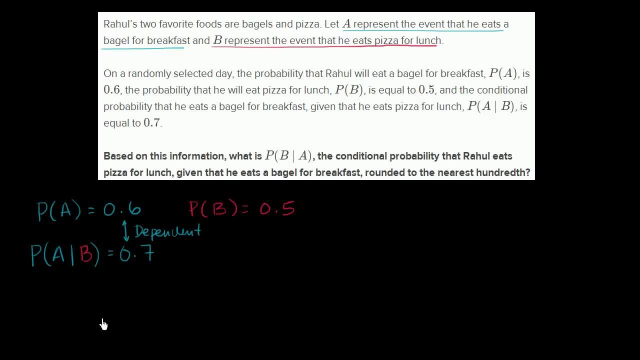 Dependent. And so when we start thinking- well, actually, let's, just before I start going on my little soapbox about dependent events, let's just think about what they actually want us to figure out. So the probability, the probability that he eats. 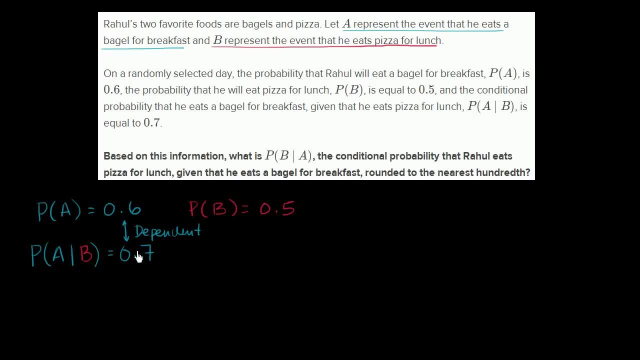 the probability of A given B is equal to 0.7,. that's what we wrote right over here. Based on this information, what is the probability of B given A? So they want us to figure out the probability of B given. 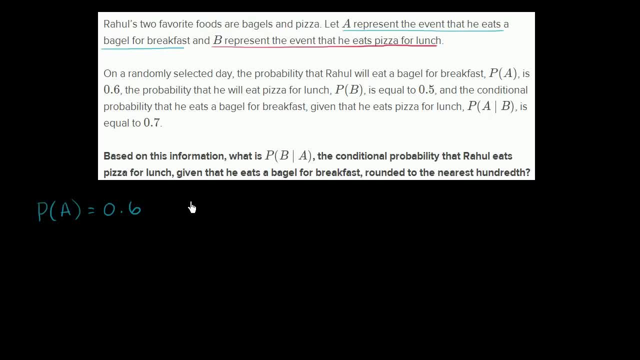 let me do that in that red color. the probability of event B that he eats a pizza for lunch is 0.5.. And the conditional probability that he eats a bagel for breakfast. given that he eats a bagel for breakfast, 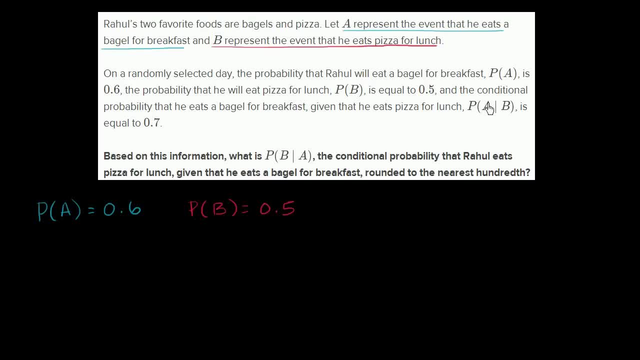 is a pizza for lunch, so probability of event A happening that he eats a bagel for breakfast, given that he's had a pizza for lunch, is equal to 0.7, which is interesting, So let me write this down. 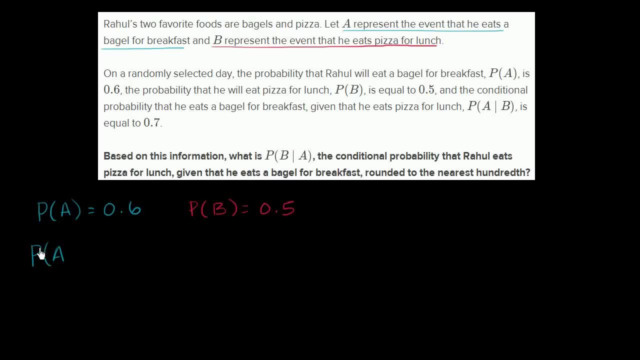 The probability of A, given that B is true, given B is not 0.6, it's equal to 0.7.. And because these two things are not the same, because probability of A by itself is different than the probability of A. 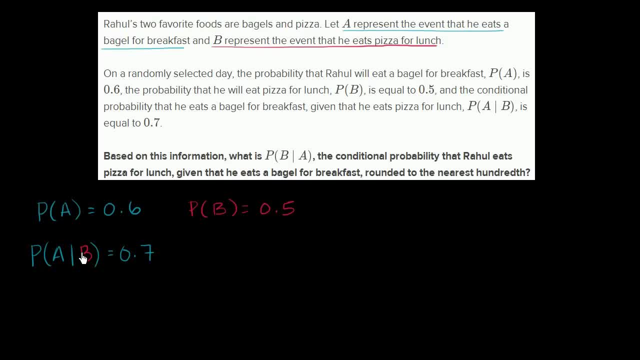 given that B is true. this tells us that these two events are not independent, that we're dealing with dependent probability. This shows us the fact that B being true has changed the probability of A being true. This tells us that A and B are dependent. 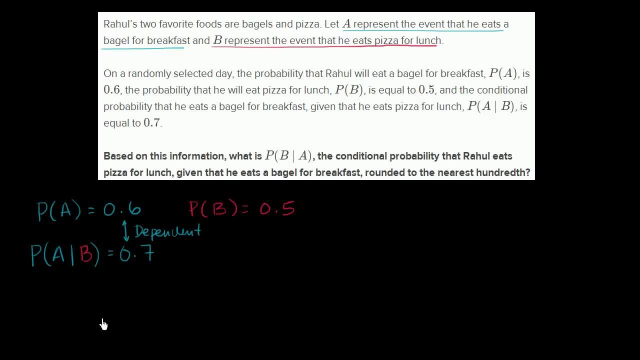 Dependent. And so when we start thinking- well, actually, let's, just before I start going on my little soapbox about dependent events, let's just think about what they actually want us to figure out. So the probability, the probability that he eats. 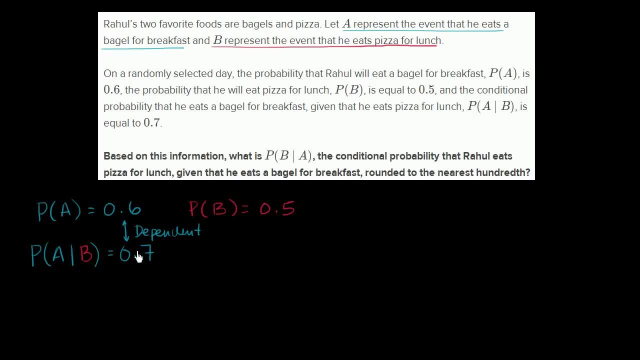 the probability of A given B is equal to 0.7,. that's what we wrote right over here. Based on this information, what is the probability of B given A? So they want us to figure out the probability of B given. 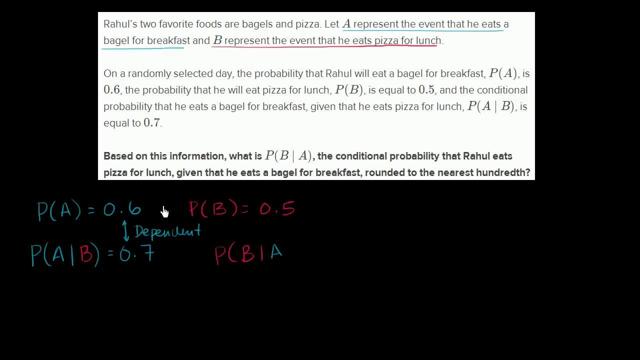 probability of B given A- That's what they want us to figure out- The conditional probability that Rahul eats pizza for lunch, given that he eats a bagel for breakfast, rounded to the nearest hundredth. So how would we think about this? 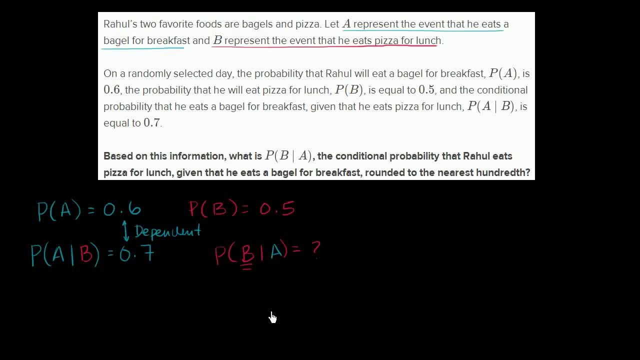 And I encourage you to pause this video before I work through it. So I'm assuming you've given a go at it. So the best way to tackle this is to just think about: well, what's the probability that both A and B are going to happen? 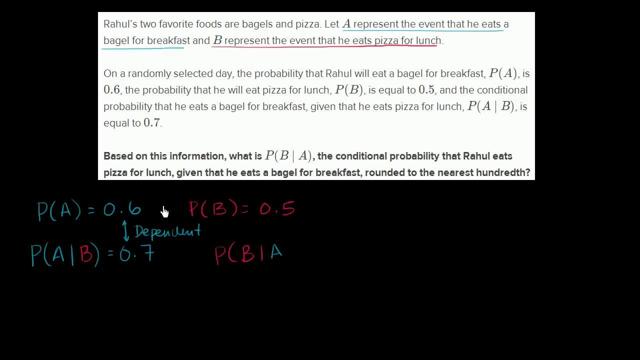 probability of B given A- That's what they want us to figure out- The conditional probability that Rahul eats pizza for lunch, given that he eats a bagel for breakfast, rounded to the nearest hundredth. So how would we think about this? 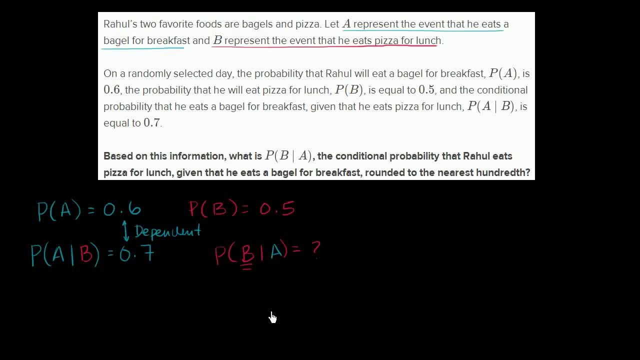 And I encourage you to pause this video before I work through it. So I'm assuming you've given a go at it. So the best way to tackle this is to just think about: well, what's the probability that both A and B are going to happen? 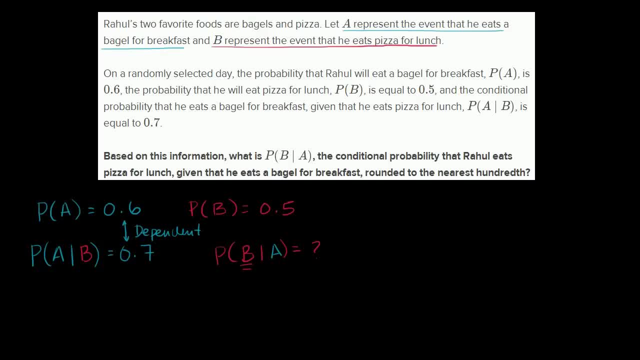 Well, the probability of A and B happening- let me do this in a new color. the probability of A and B happening- A and B- I want to stay true to the colors- is equal to. there's a couple of ways you could write this out. 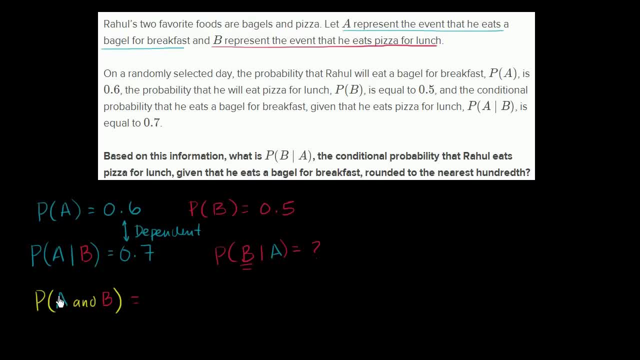 This is equivalent to. this is equivalent to the probability probability of A given B, given B times the probability of B, and hopefully that makes sense: A, the probability that B happens and that, given that B has happened, the probability that A happens. 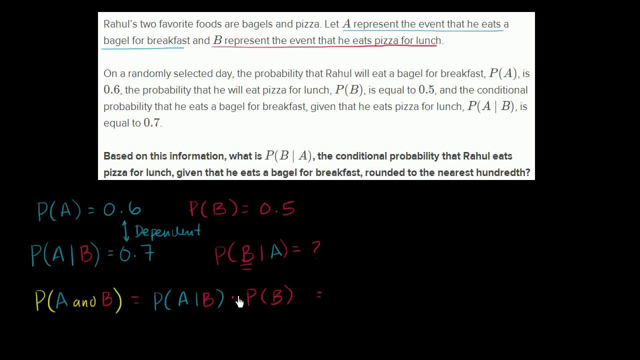 And that would also be equal to. so obviously this is A and B is happening, or you could do it the other way around. You could view it as the probability that B, the probability that B given A happens, given A happens, times the probability of A. 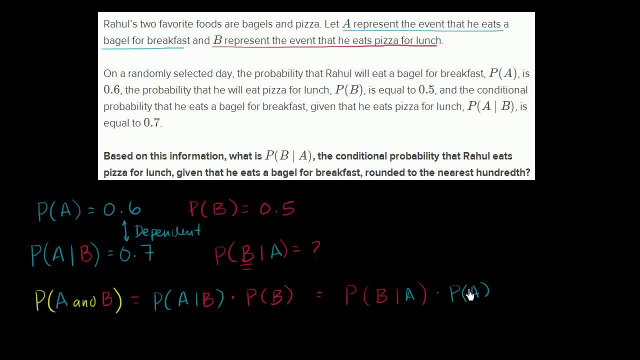 times the probability of A. This also makes sense. What's the probability that A happened And that, given A happened, what's the probability of B? You multiply those together, you get the probability that both happened. So why is this helpful for us? 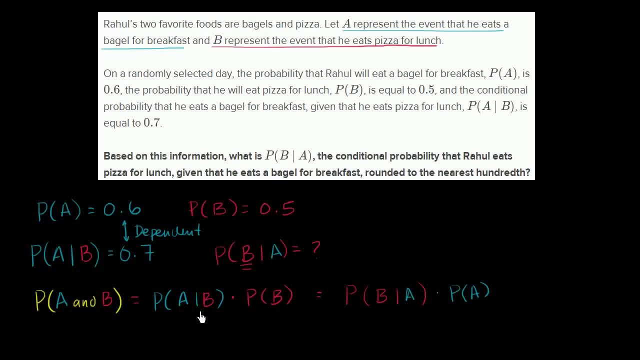 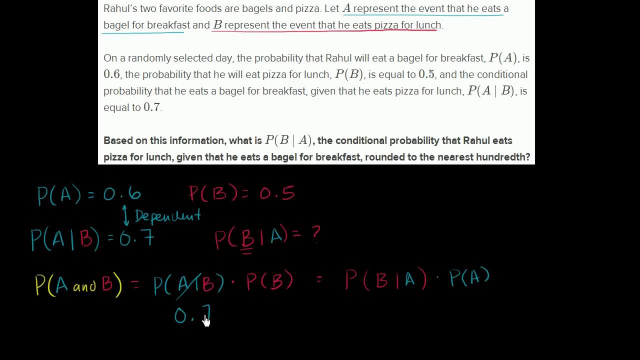 Well, we know a lot of this information. We know the probability of A given B is 0.7.. So let me write this. I'll scroll down a little bit: This is 0.7.. We know that the probability of B is 0.5.. 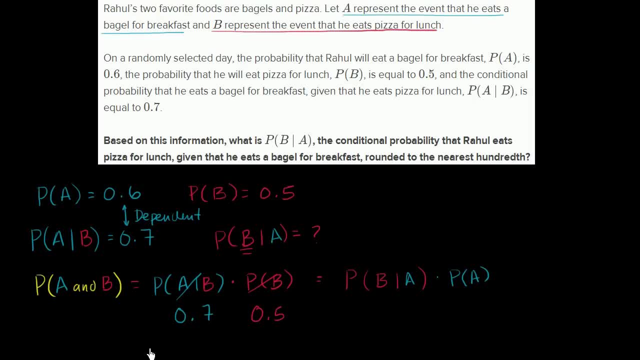 So this is 0.5.. So we know that the probability of A and B is the product of these two things. That's going to be 0.35.. Seven times five is 35. Or I guess you could say half of 0.7 is 0.35.. 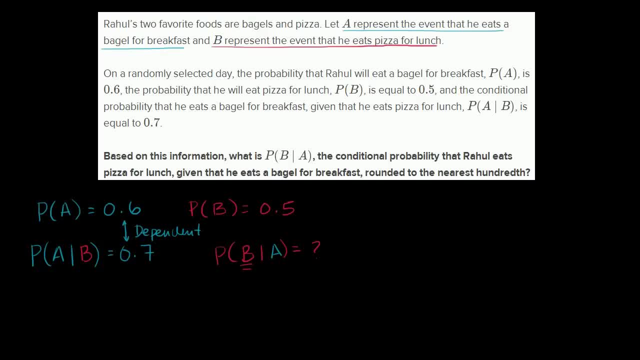 Well, the probability of A and B happening- let me do this in a new color. the probability of A and B happening- A and B- I want to stay true to the colors- is equal to. there's a couple of ways you could write this out. 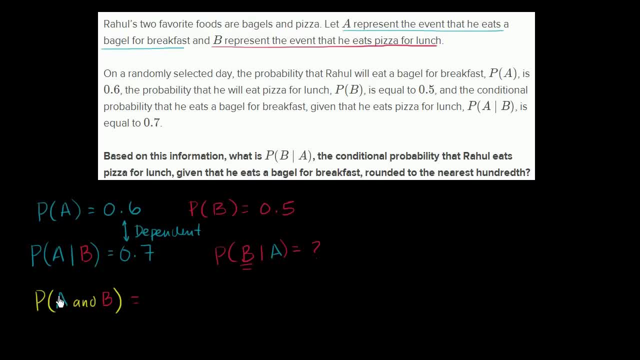 This is equivalent to. this is equivalent to the probability probability of A given B, given B times the probability of B, and hopefully that makes sense: A, the probability that B happens and that, given that B has happened, the probability that A happens. 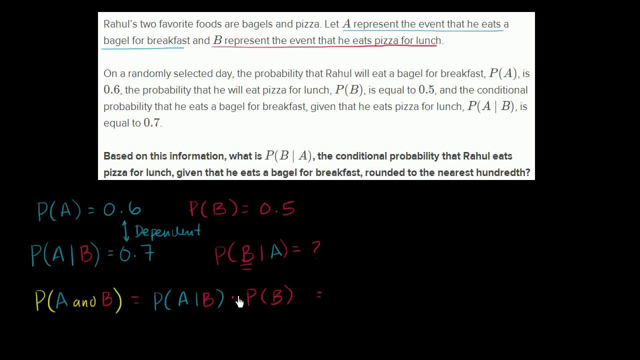 And that would also be equal to. so obviously this is A and B is happening, or you could do it the other way around. You could view it as the probability that B, the probability that B given A happens, given A happens, times the probability of A. 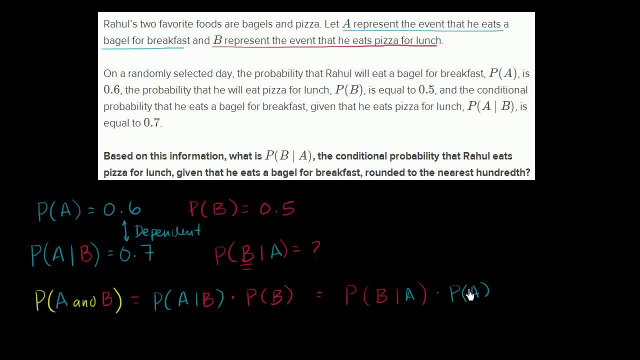 times the probability of A. This also makes sense. What's the probability that A happened And that, given A happened, what's the probability of B? You multiply those together, you get the probability that both happened. So why is this helpful for us? 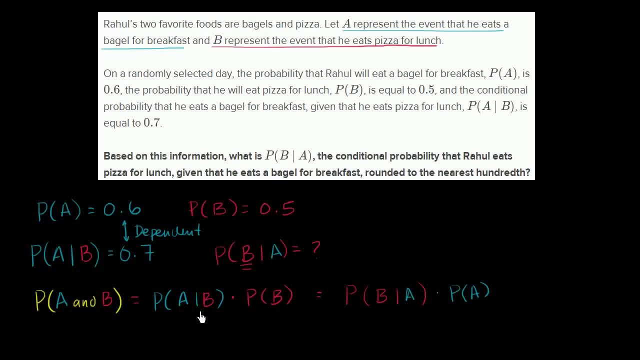 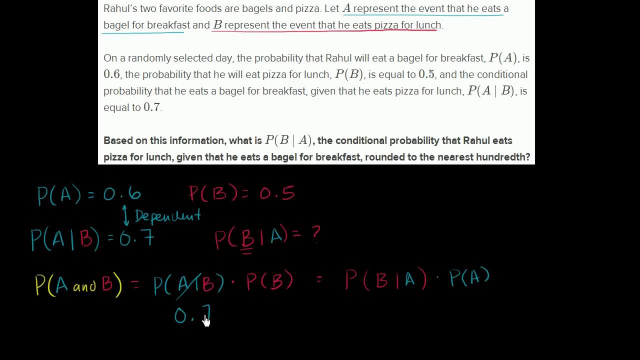 Well, we know a lot of this information. We know the probability of A given B is 0.7.. So let me write this. I'll scroll down a little bit: This is 0.7.. We know that the probability of B is 0.5.. 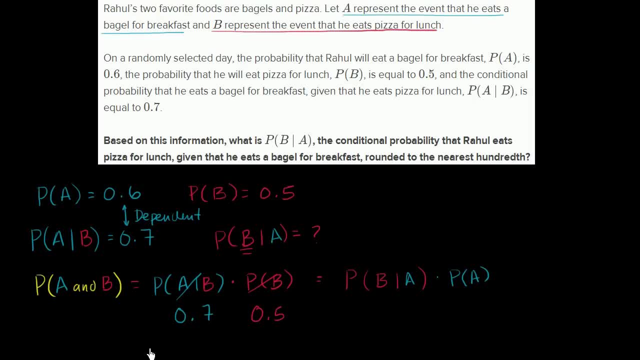 So this is 0.5.. So we know that the probability of A and B is the product of these two things. That's going to be 0.35.. Seven times five is 35. Or I guess you could say half of 0.7 is 0.35.. 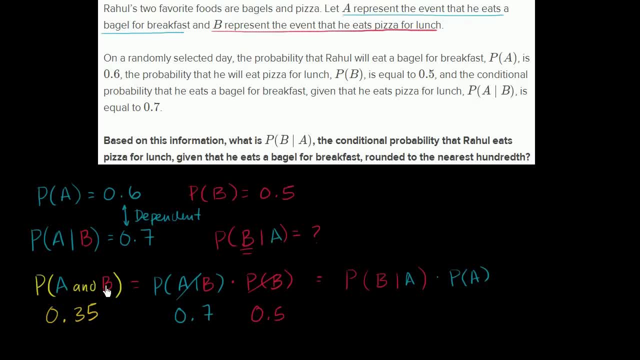 0.5 of 0.7.. And that is going to be equal to what we need to figure out: the probability of B given A times the probability of A. But we know the probability of A, We know that that is 0.6.. 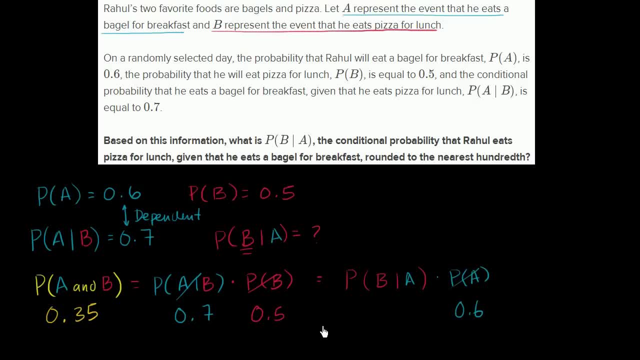 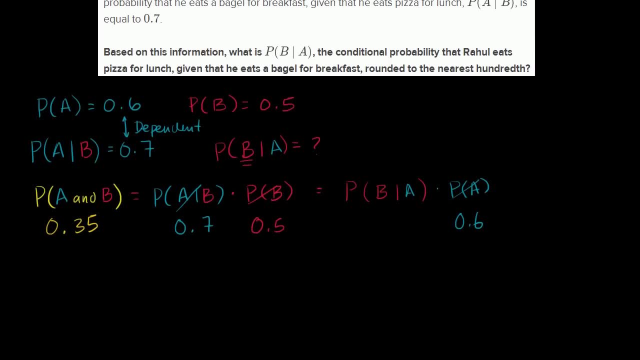 We know that this is 0.6.. So, just like that, we've set up a situation, an equation, where we can solve for the probability of B given A, The probability of B given A. notice, let me just rewrite it right over here: